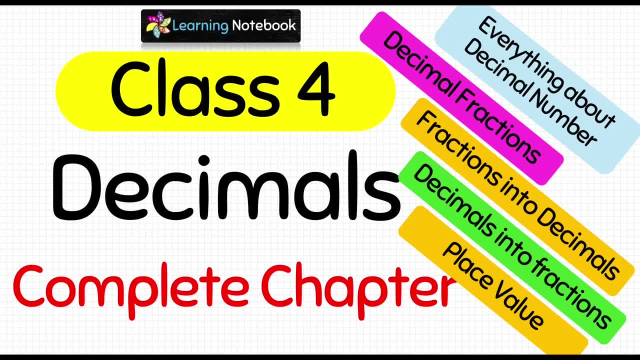 this topic. let me tell you that we have made videos on every chapter of class 4 mathematics. We also have interesting worksheets and quizzes on each chapter. You can find them on our channel, Learning Notebook. Also, you can see a list of all such videos on our website, The link to our 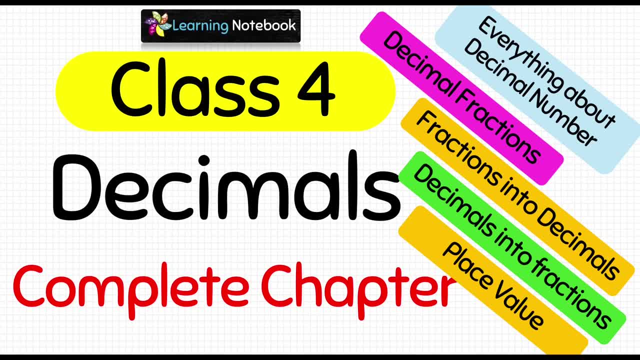 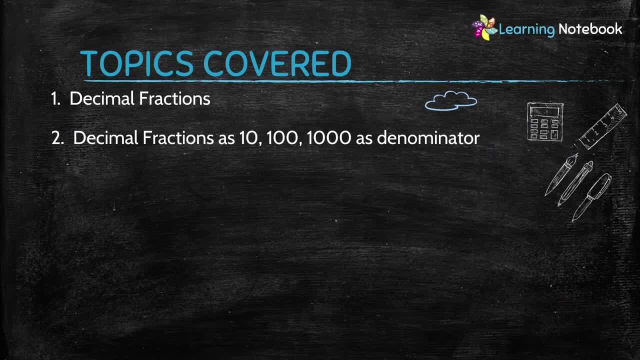 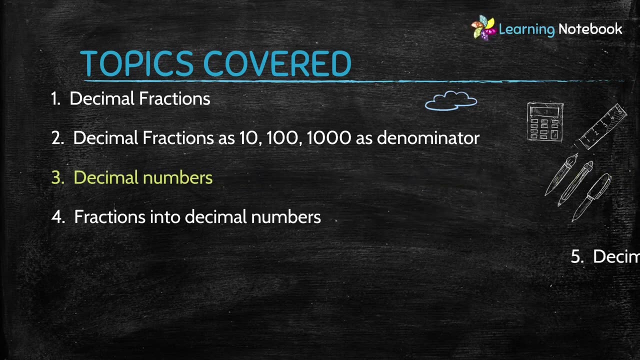 website is below in the description box. So let's see what all topics we are going to cover today in this video. First we will understand what are decimal fractions. Then we will learn about decimal fractions as 10, 100 and 1000 as denominator. After that we will learn about 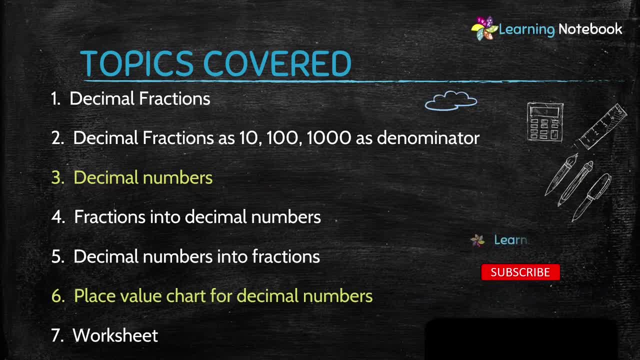 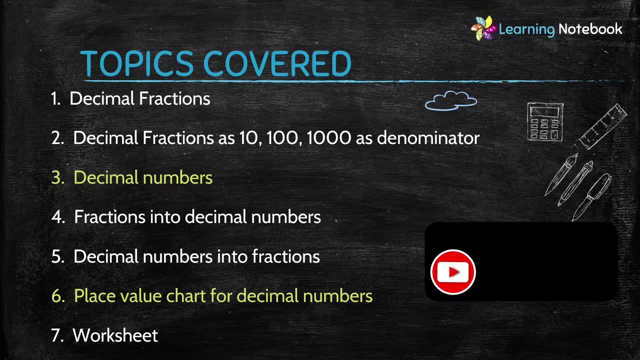 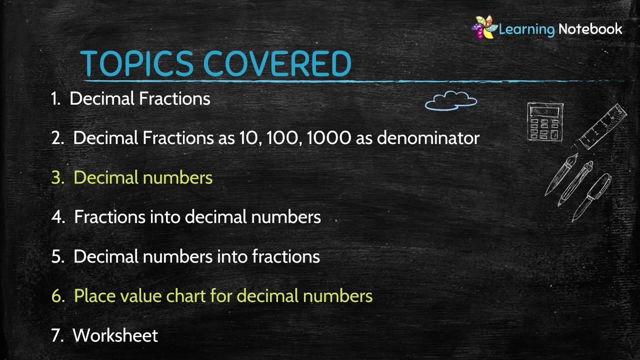 decimal numbers, how to convert fractions into decimal numbers and how to convert fractions into decimal numbers and how to convert decimal numbers into fractions. Later on we will understand place value chart for decimal numbers And in the end I will give you a worksheet on decimal numbers. 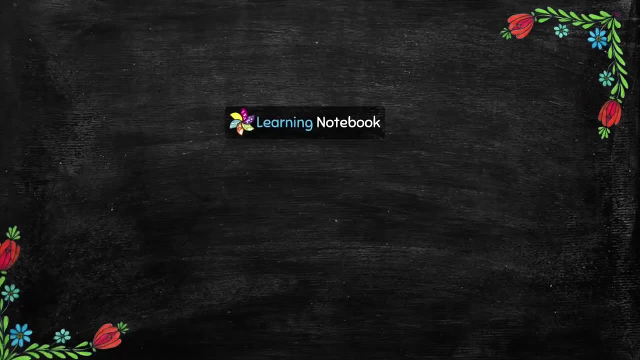 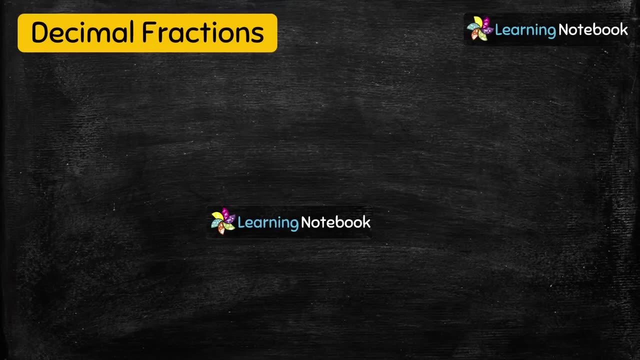 for your practice. So let's start and first understand decimal fractions. So let's start and first understand decimal fractions, Students. we have 10,, 100 and 1000 as denominator, So let's start and first understand decimal fractions. 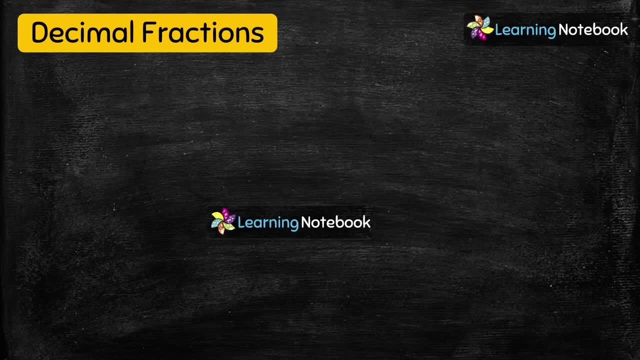 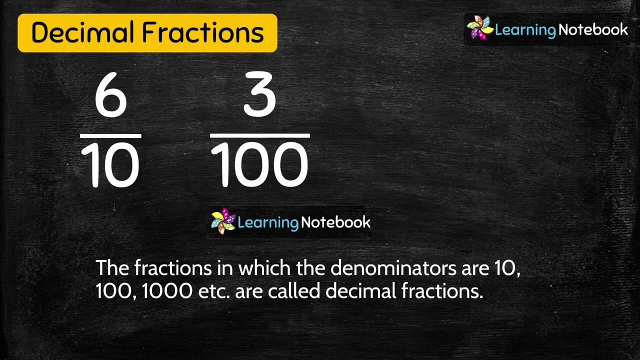 We have already learnt fractions in the previous chapter. Now we are going to use the concept of fractions in this chapter as well. But we are going to consider only those fractions which have denominators as 10, 100 or 1000. And such fractions are called. 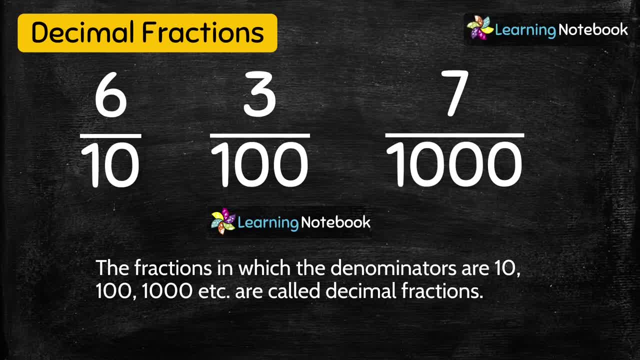 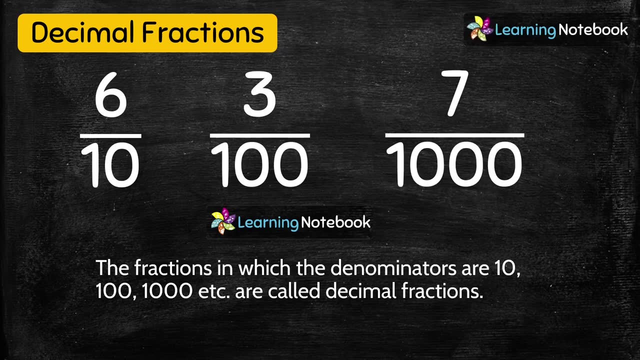 decimal fractions, For example, 6 by 10,, 3 by 100 and 7 by 1000.. These fractions have denominators 10, 100 and 1000.. So these are called as decimal fractions. So let's start and first understand decimal fractions. 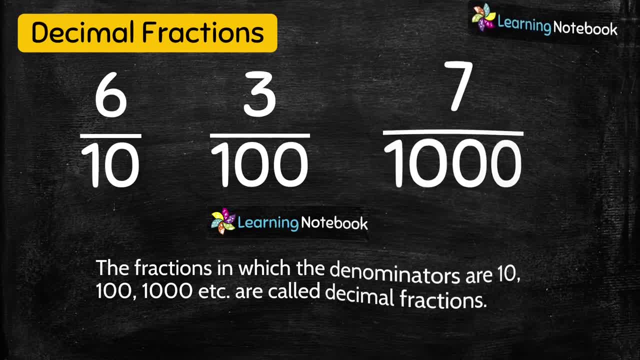 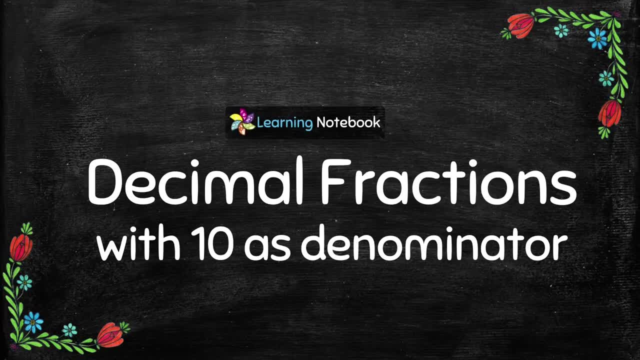 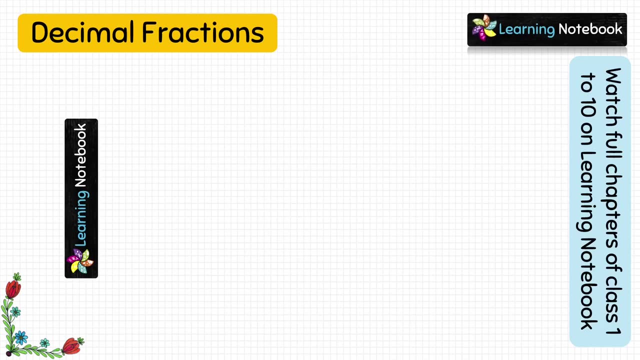 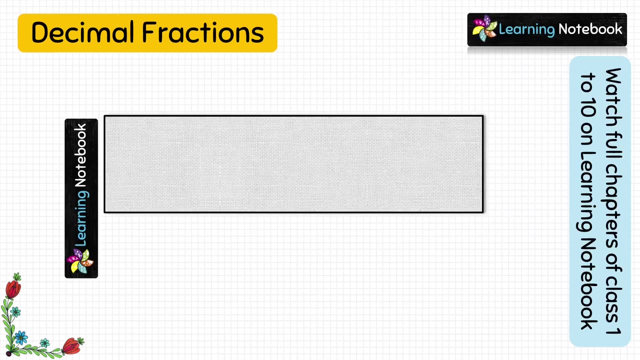 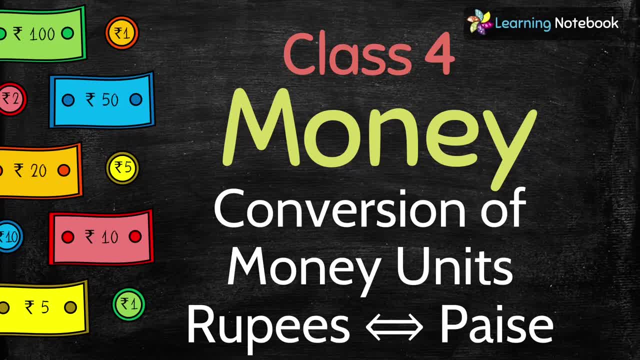 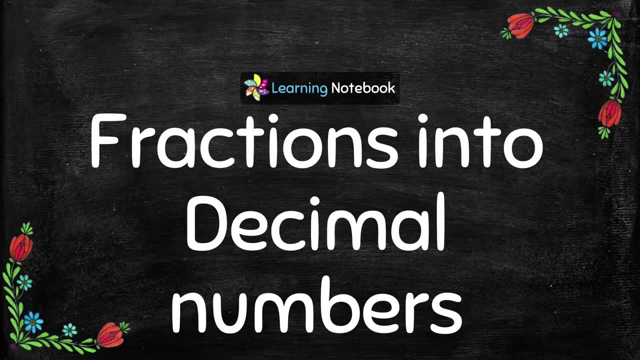 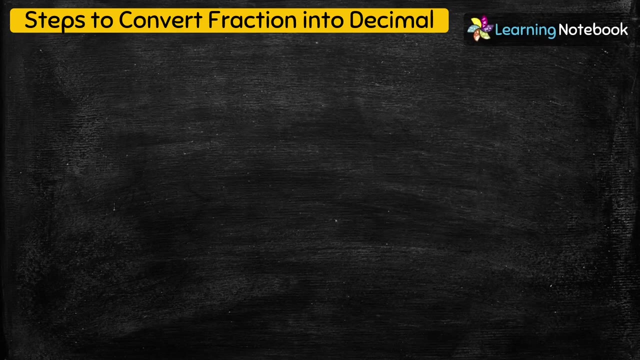 Students, we have a separate video on complete chapter of money for class 4.. The link to this video is below in the description box. Now our next topic is how to convert fractions into decimal numbers. Again, students, we have to follow some steps to convert fraction into decimal. 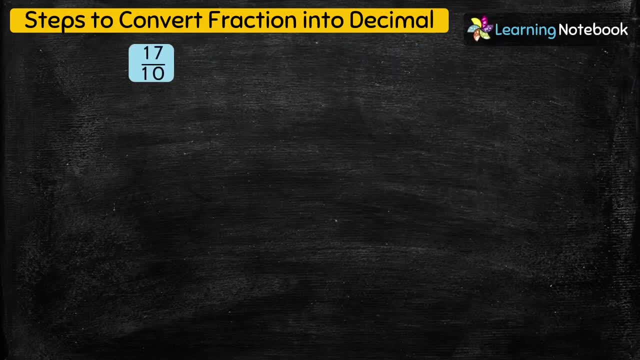 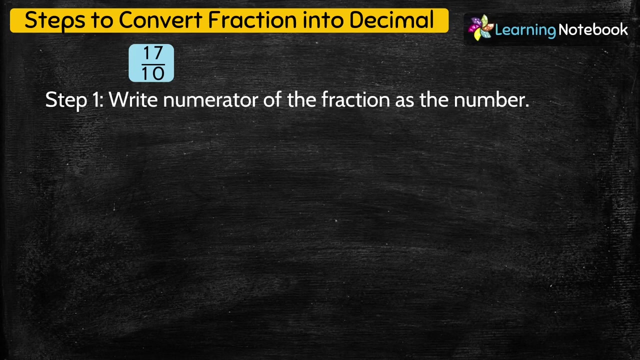 So let's take an example and understand these steps side by side. Question is: convert fraction 17 by 10 into decimal. So in step 1, we will write numerator of the fraction as the number. So here numerator is 17.. 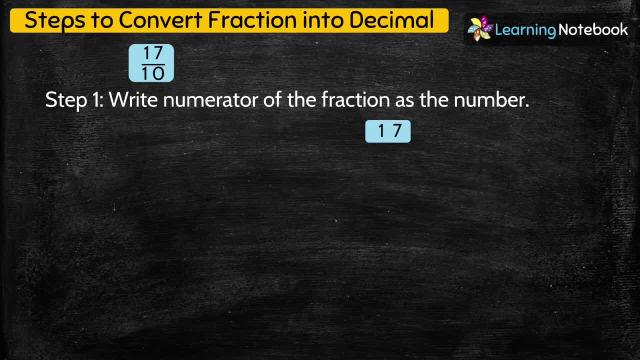 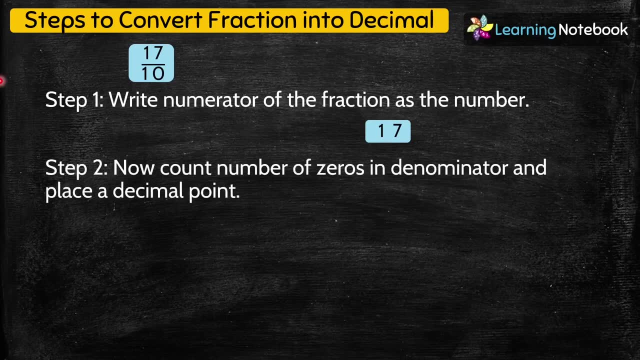 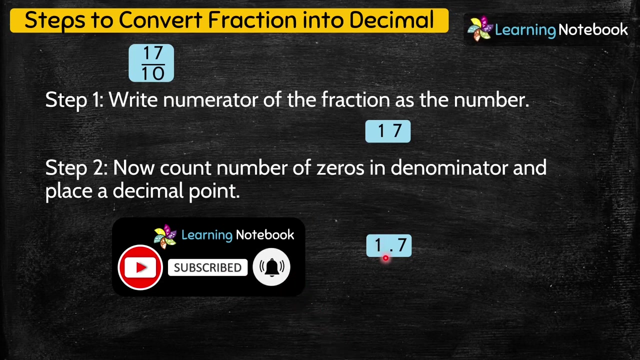 So we will write 17 as the number. Now in step 2, we will count number of zeros in the denominator and place the decimal point. So, students, here number of zero is 1.. So we will put decimal at one decimal place. 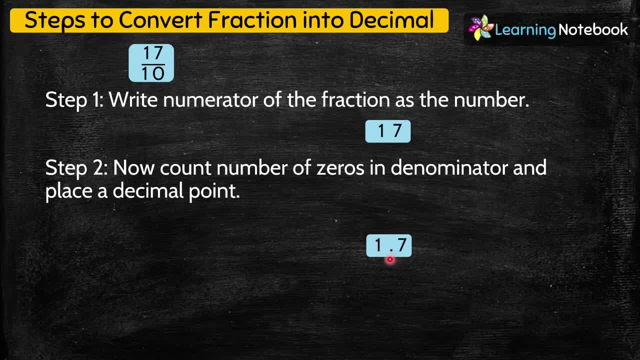 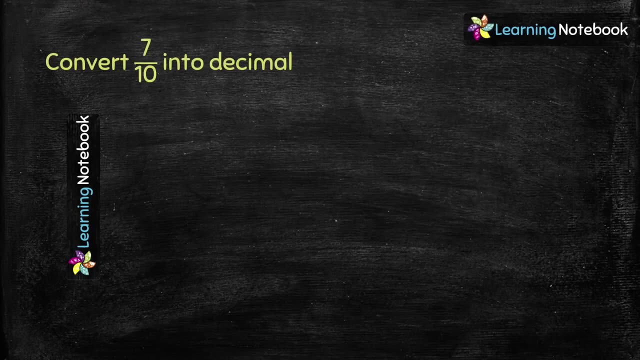 That is, we will write the number as 1.7.. So in this way we have converted fraction into decimal 1.7.. Question is: convert 7 by 10 into decimal. So, students, first we will write the numerator of the fraction as the number. 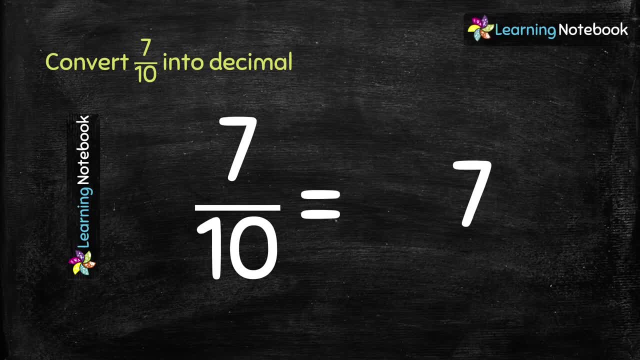 So numerator is 7.. So let's write the number as 7.. Then we will count number of zeros in the denominator. As we can see, there is only one zero in the denominator. So let's place a decimal point at one decimal place. 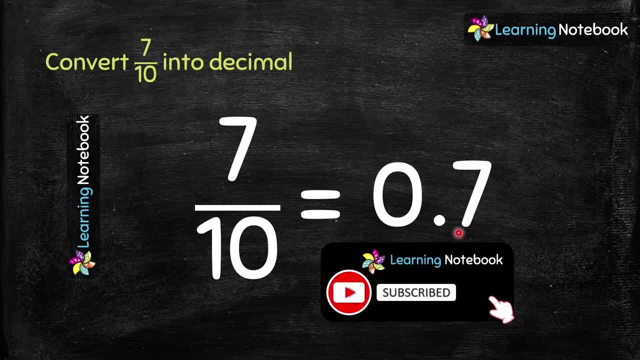 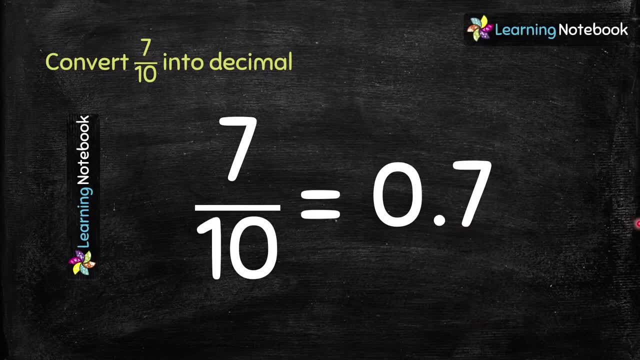 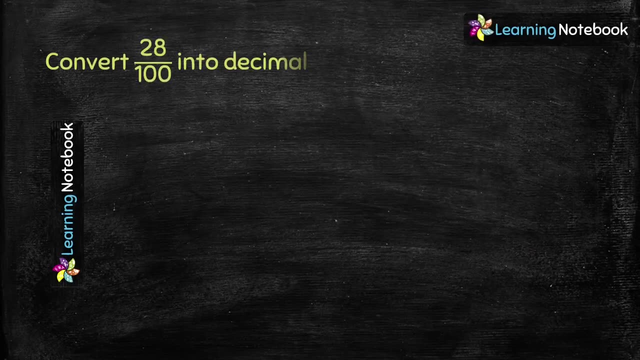 So we have got the answer as 0.7.. So we have converted fraction 7 by 10 into decimal 0.7.. Let's see the next question. Convert 28 by 100 into decimal, So here numerator is 28.. 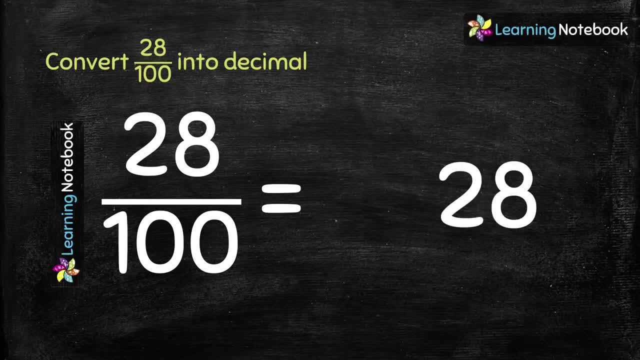 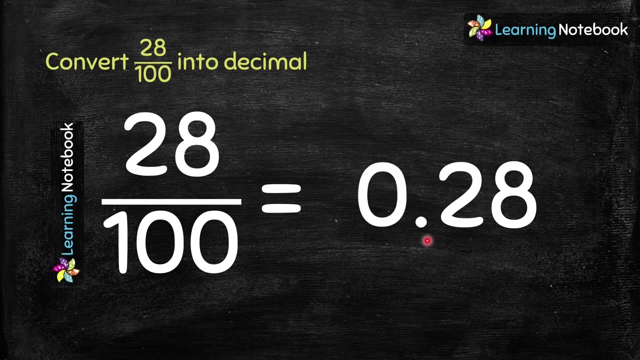 So we will write 28.. And then we can see there are two zeros in the denominator. So let's place a decimal point at two decimal places. So we will count from right 1, 2 and put the decimal point. So answer is 0.28. 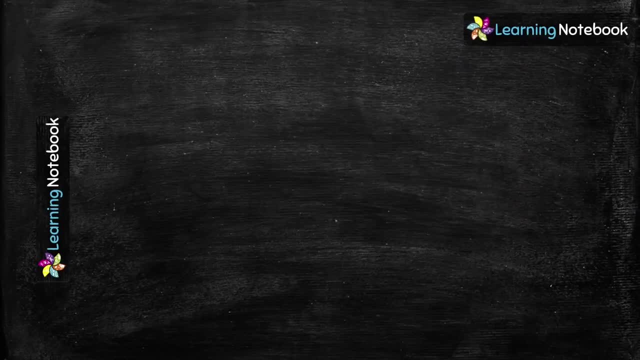 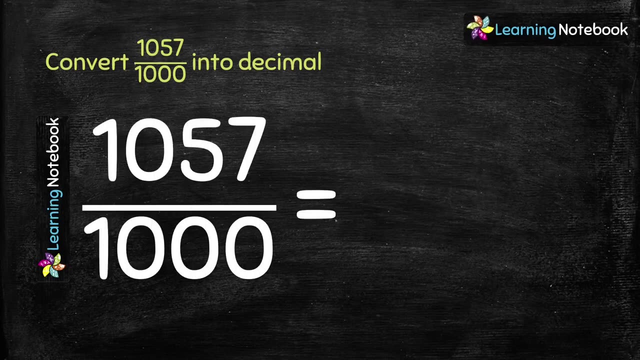 Now the next question is: convert 1057 by 1000 into decimal. So first we will write the numerator 1057 as the number. Now there are three zeros in the denominator, So we will put a decimal point at three decimal places. 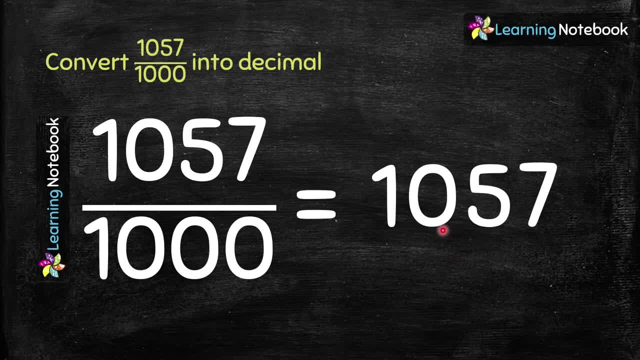 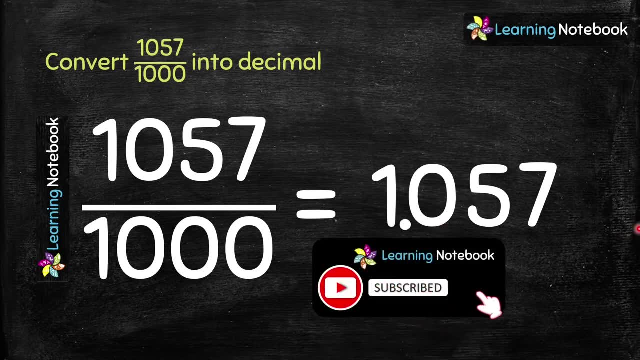 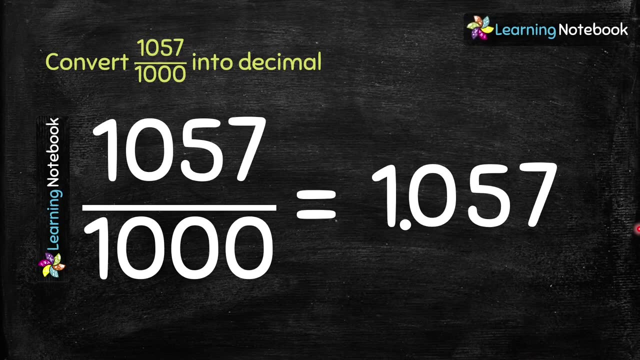 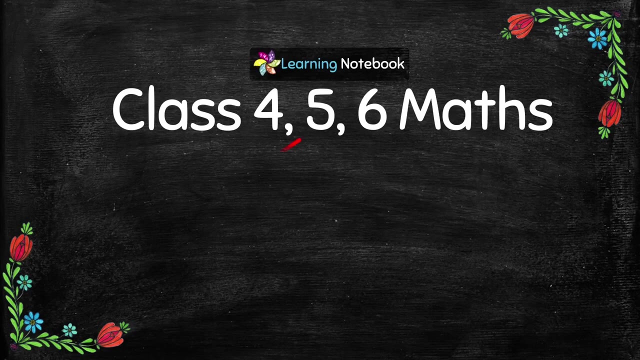 So count from right 1,, 2,, 3 and put a decimal point here, So we have got the answer as 1.057.. So, students, this is how we convert a fraction into decimal. Students, we would like to tell you that we have made videos on every chapter of class 4, class 5 and class 6 mathematics. 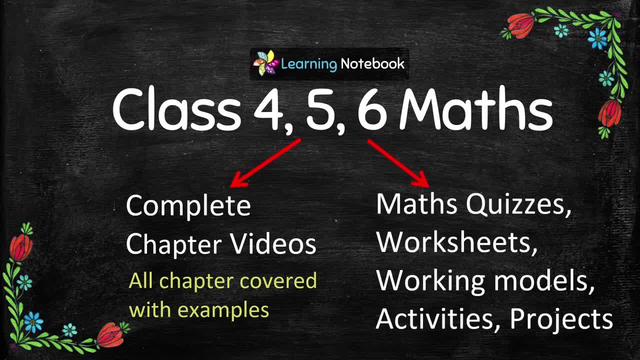 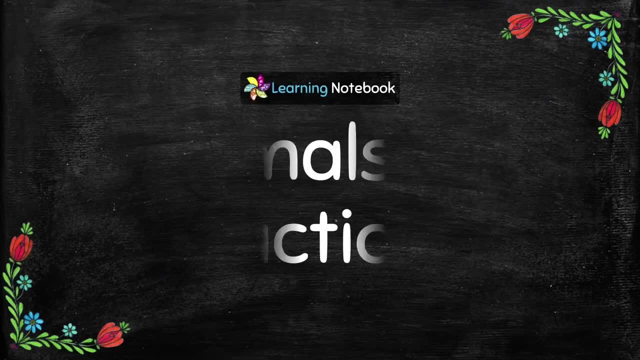 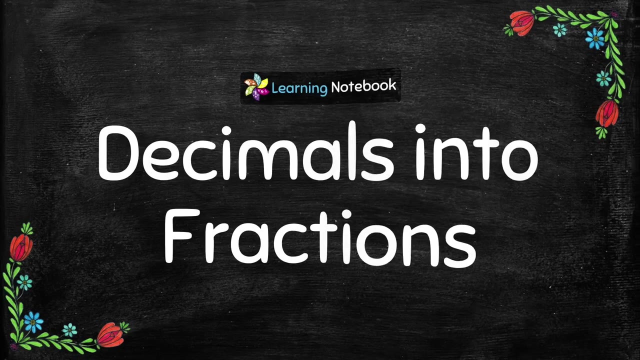 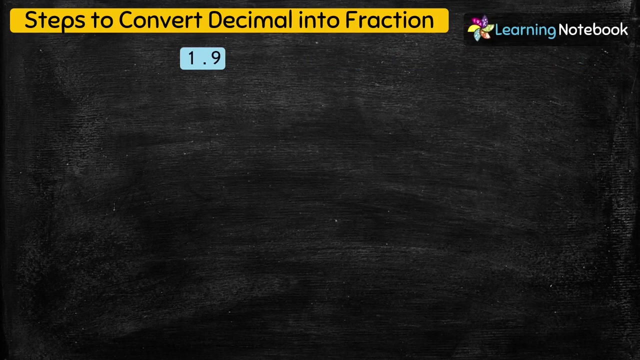 We also have interesting maths quizzes, worksheets, working modules, activities and projects on each chapter, So I would suggest you to check out our channel Learning Notebook. Now, students, let's learn how to convert decimals into fractions. We need to follow some steps to convert decimal into fraction. 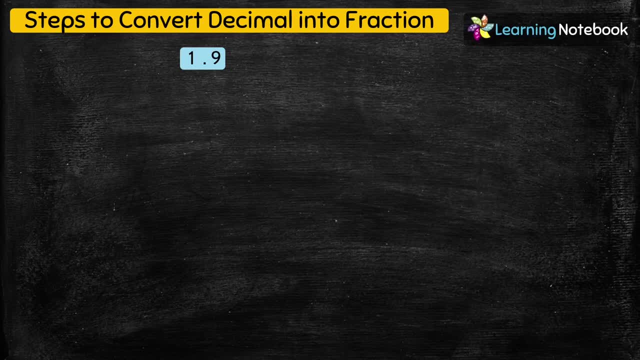 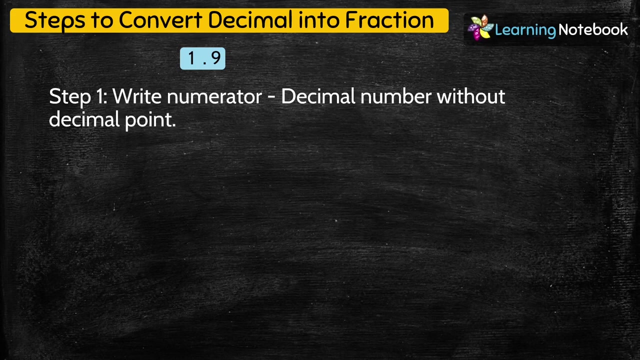 So let's take an example and follow these steps to convert. So here question is: Convert 1.9 into fraction. So in step 1, we will write the numerator of the fraction, which is the given decimal number without decimal point. So numerator of this fraction would be 19.. 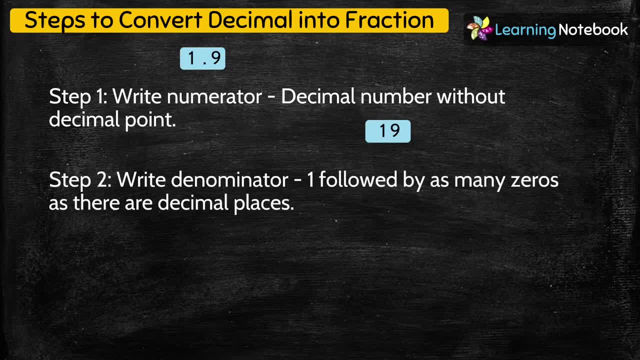 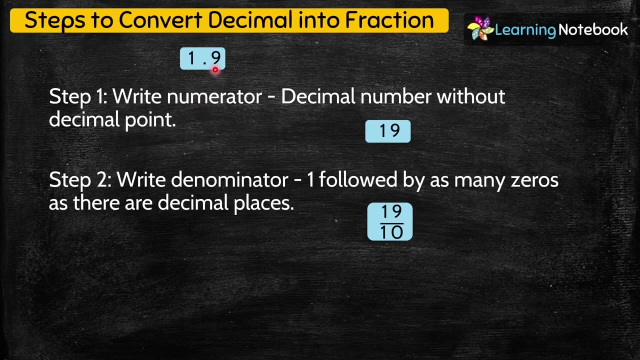 In step 2, we will write the denominator of the fraction, which is 1, followed by as many zeros as there are decimal places in the given decimal number. So, students, here decimal place is only 1.. So we will write 1, followed by 10.. 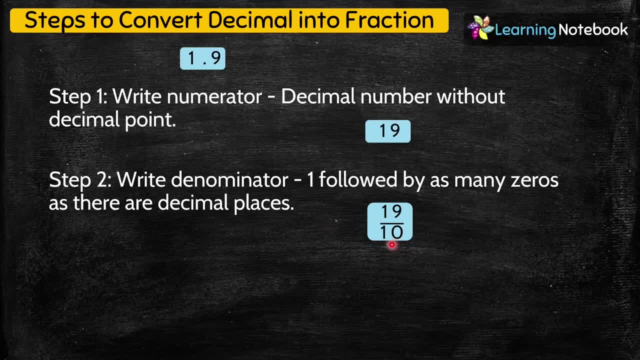 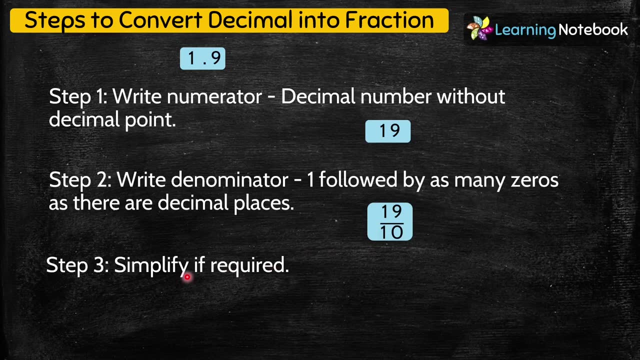 So we get the denominator of the fraction as 10.. So we have converted the given decimal into fraction 19 upon 10.. And in step 3, we will simplify if required. But here we are not going to simplify it because there is no common factor between numerator and denominator. 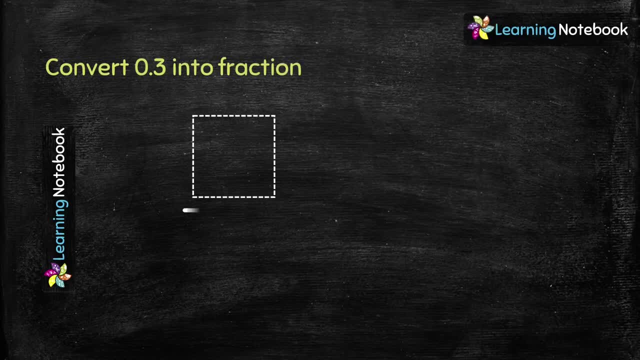 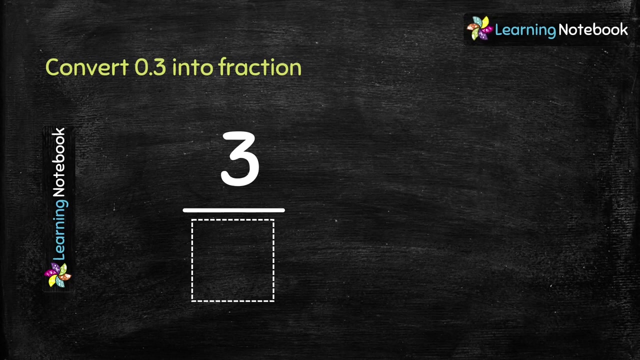 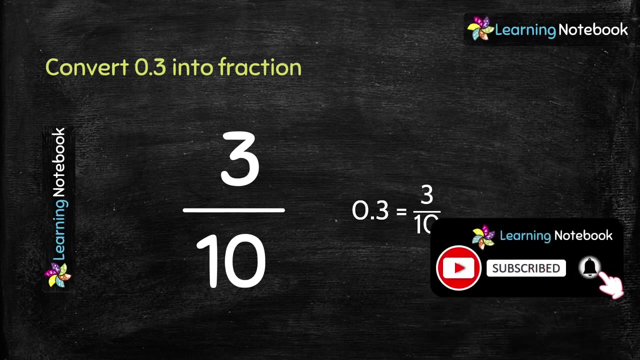 Now let's do another question: Convert 0.3 into fraction. So, students, first let's write the numerator, which is 3.. Now this decimal number has only 1 decimal place, So its denominator will be 10.. So we have converted 0.3 into fraction 3 by 10.. 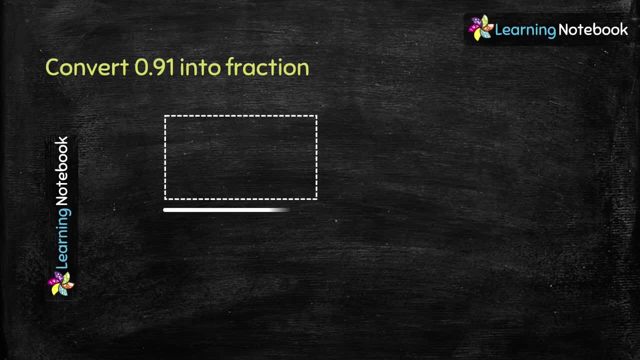 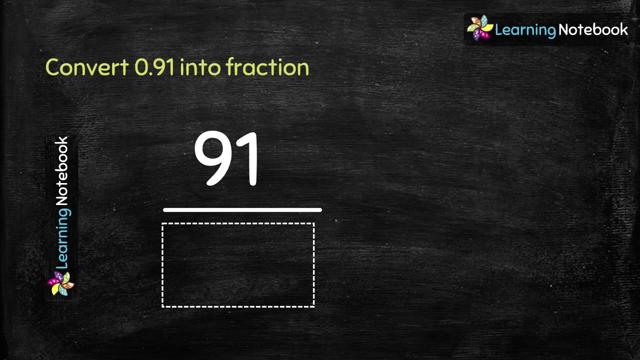 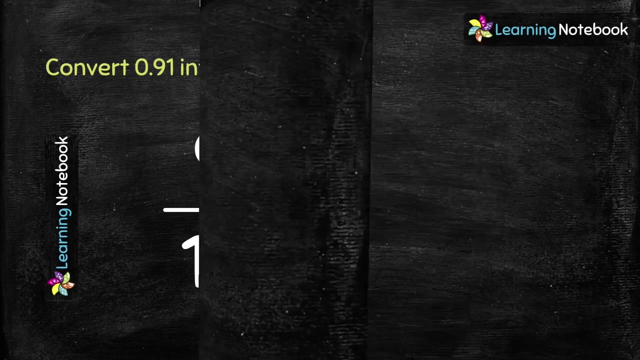 Next question is: Convert 0.91 into fraction. Let's first write the numerator, which is 91.. Now this decimal number has how many decimal places? 2.. So its denominator will be 100.. So we have converted 0.91 into fraction 91 by 100.. 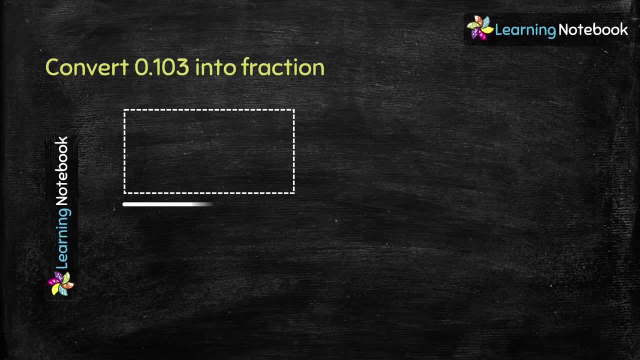 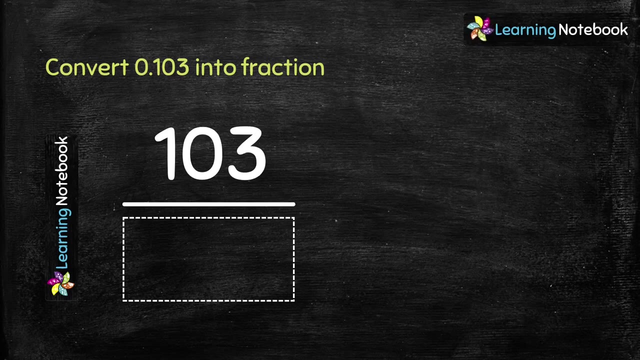 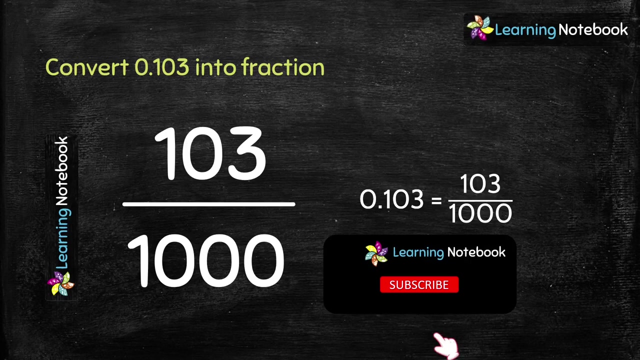 Now our next question is: Convert 0.103 into fraction, So the numerator will be 103.. And this decimal number has 3 decimal places, So its denominator will be 1000.. So we have converted the decimal number 0.103. 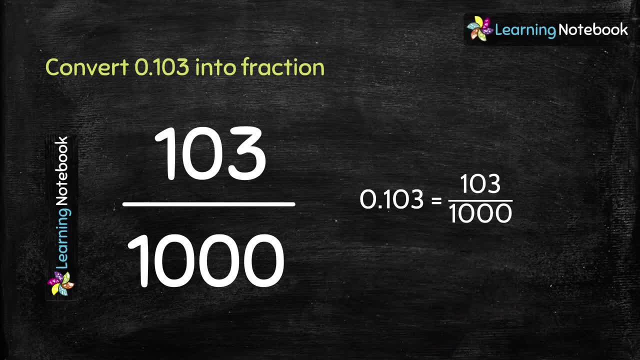 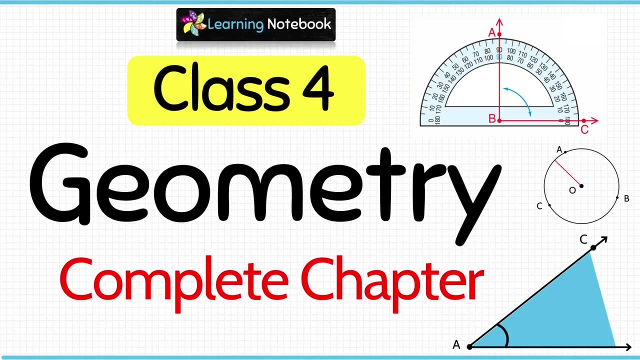 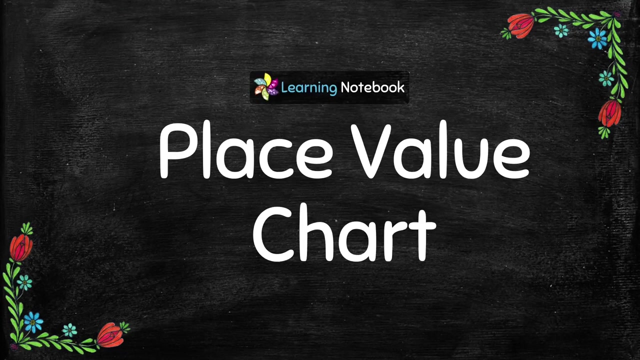 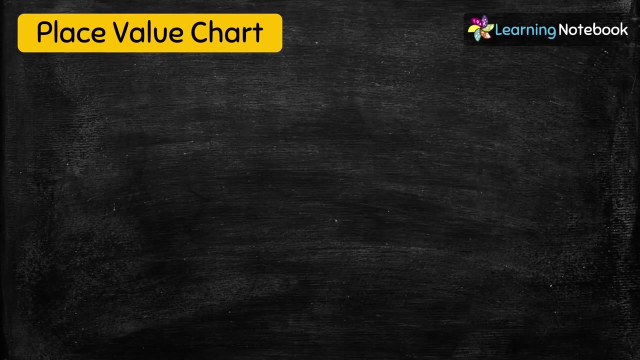 into fraction 103 by 1000.. To learn concepts of geometry for class 4, you can refer to our separate video. You will find its link below in the description box. Now let's understand place value chart of a decimal number. Place value chart for whole number. part remains the same. 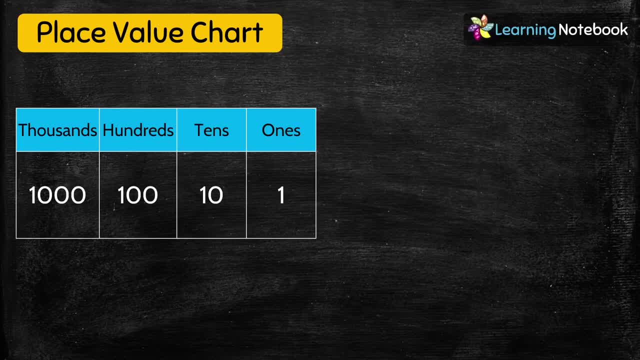 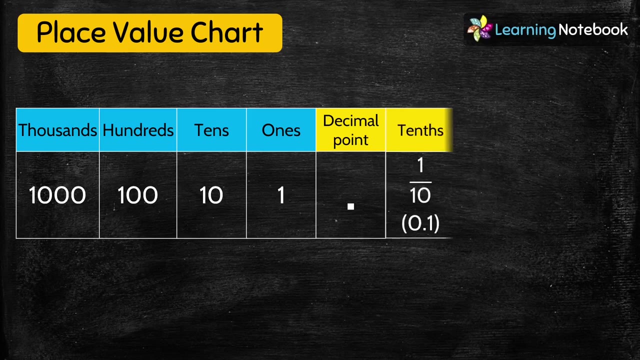 Which is 1s, 10s, 100s, 1000s and so on. Next we have decimal point, And then there is 10s, Which is 1 by 10 or 0.1.. After that there is 100s place. 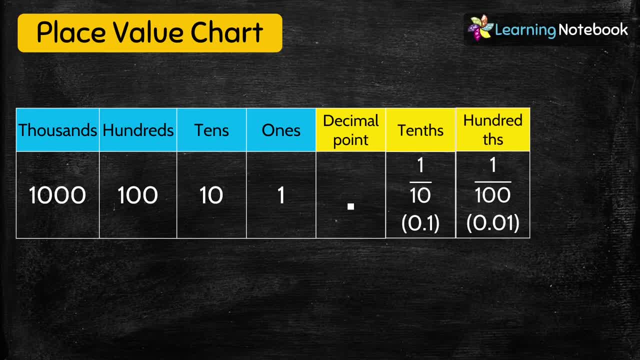 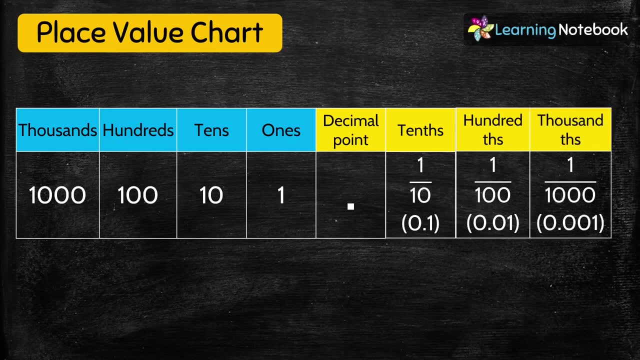 Which is 1 by 100 or 0.01.. And next is 1000s place, Which is 1 by 1000 or 0.001.. So this is the place value chart for decimal numbers. Now let's do a question on place value chart. 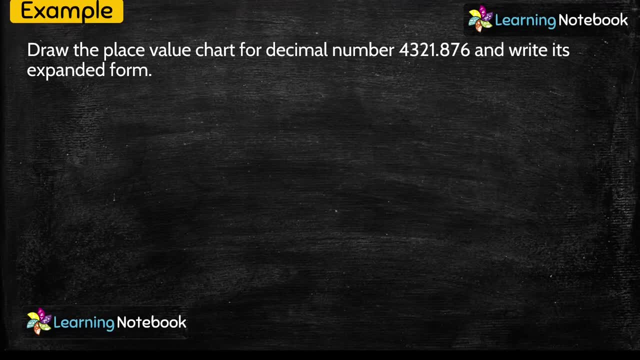 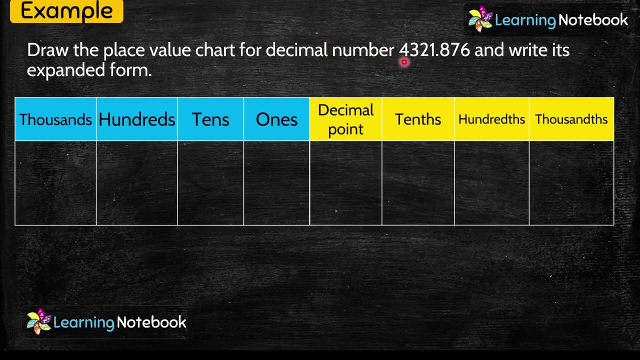 Question is: Draw the place value chart for decimal number 4321.873.. And write its expanded form. So let's draw the place value chart First. we will represent whole number part of this decimal number. Whole number part is 4321.. 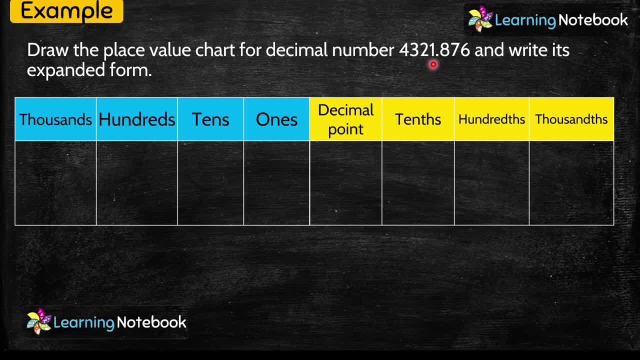 So let's represent it. 1 is at 1s place, 2 is at 10s place, 3 is at 100s place And 4 is at 1000s place. Now let's put the decimal point in the place value chart. 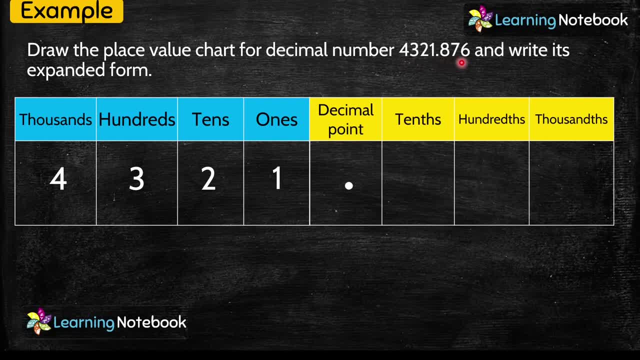 Then we will represent the decimal part, Which is 876.. Where 8 is at 10s place, 7 is at 100s place And 6 is at 1000s place. Now we need to write the expanded form of this decimal number. 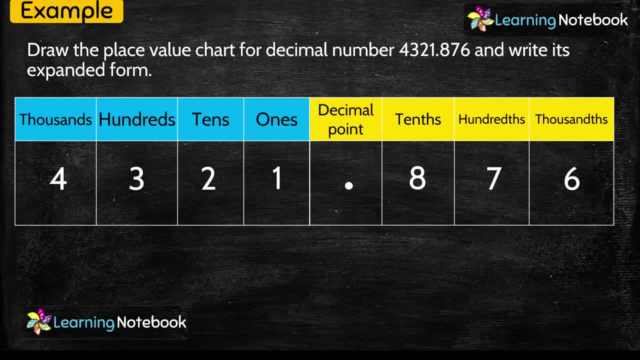 For this, first we need to find the place value of all the digits of this decimal number. So let's first write the place value of whole number part. Place value of 1 is 1.. Place value of 2 is 20.. 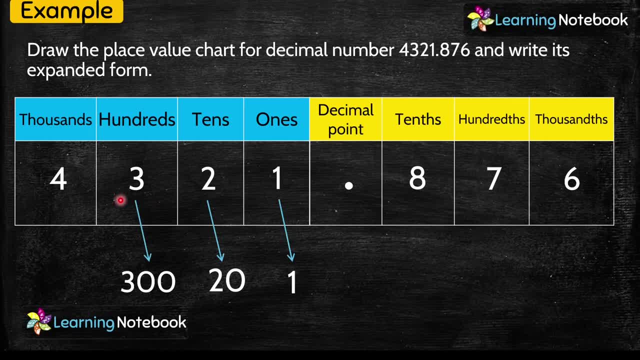 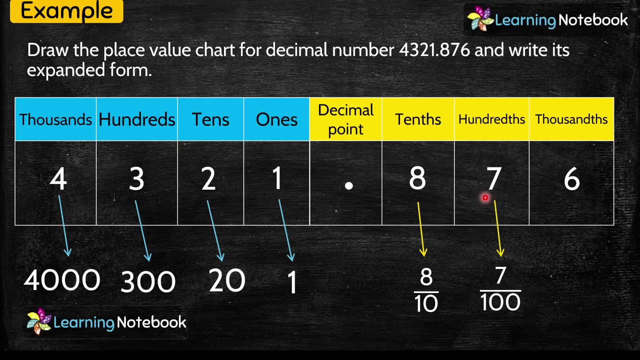 Place value of 3 is 300.. And place value of 4 is 4000.. Now let's write the place value of decimal part. Place value of 8 is 8 by 10.. Place value of 7 is 7 by 100.. 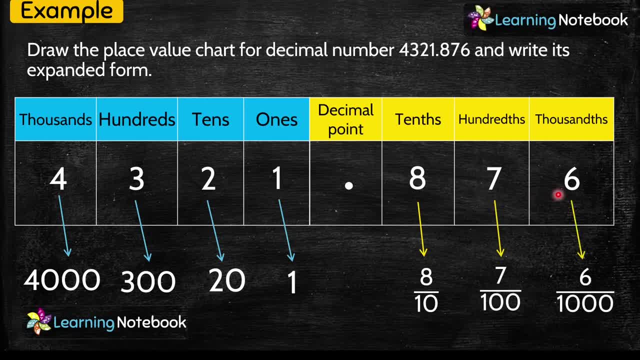 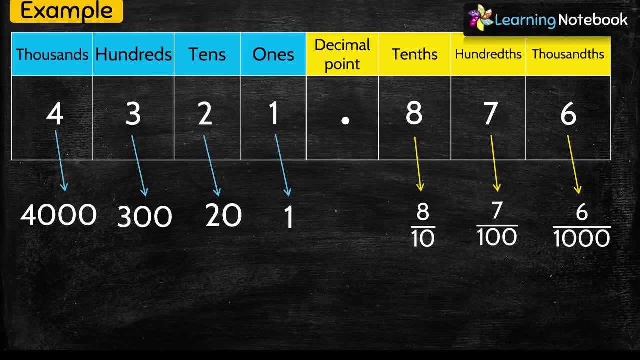 And place value of 6 is 6 by 1000.. Now, students, we know expanded form of a number is the sum of the place value of all of its digits. So let's write the expanded form of this decimal number: 4000 plus 300 plus 20 plus 1.. 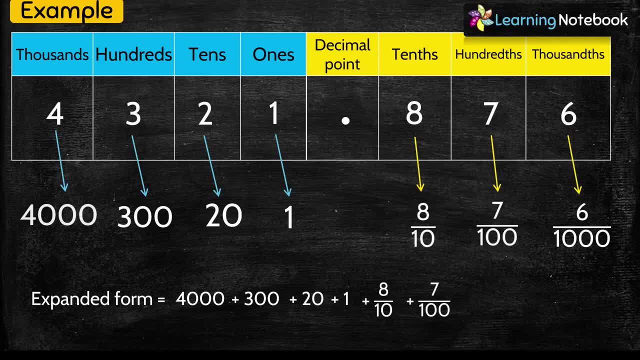 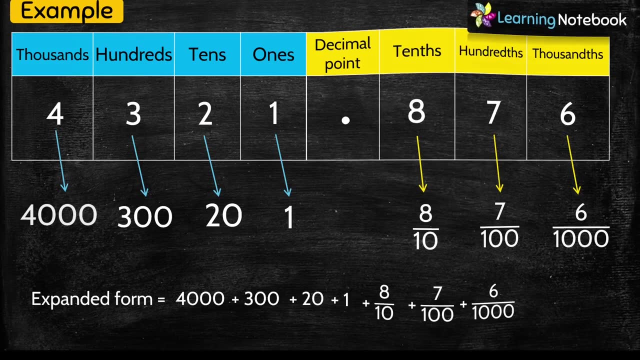 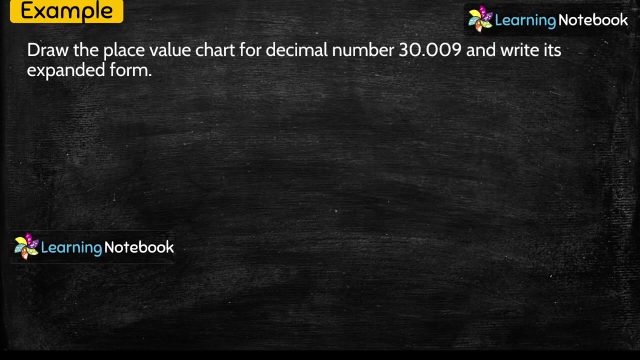 Plus 8 by 10.. Plus 7 by 100.. Plus 6 by 1000.. So this is how we write the expanded form of a decimal number. Let's do one more question. Draw the place value chart for decimal number 30.009.. 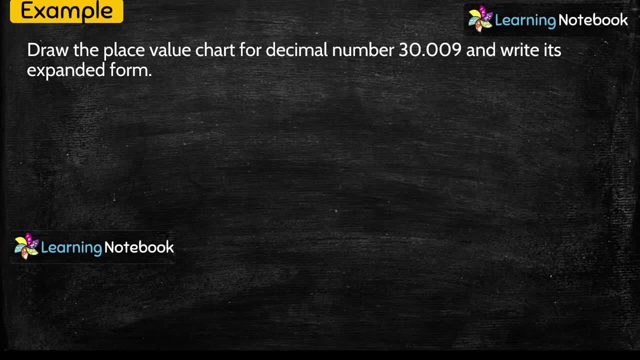 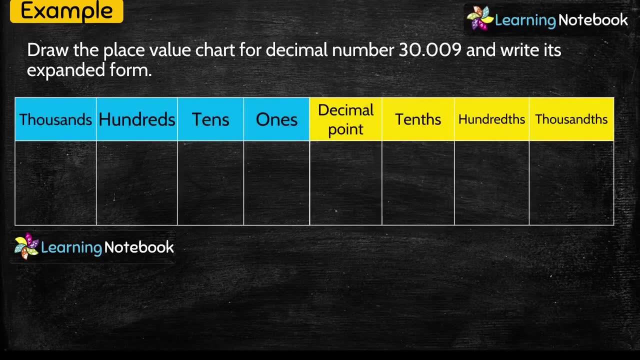 And write its expanded form. Now let's draw the place value chart And first represent the whole number part of this decimal number. Whole number part is 30. So we will write 0 at 1's place and 3 at 10's place. 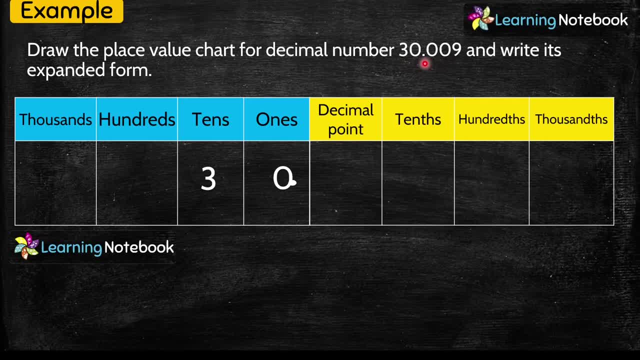 Then we will put a decimal point, Next we will represent the decimal part of this decimal number. So 0 comes at 10's place, Next 0 comes at 100's place, And then we will write 9 at 1000's place. 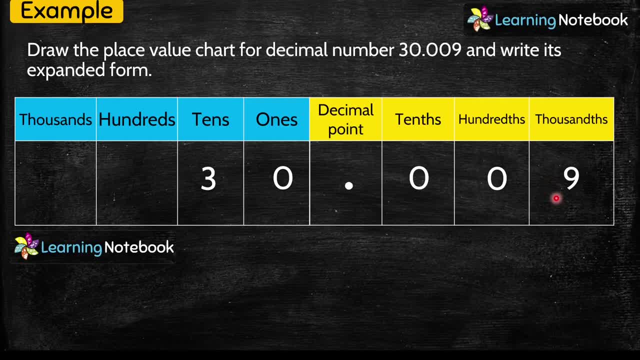 Now to write the expanded form of this decimal number, First we have to find the place value of all of its digits. So first let's write the place value of whole number part. Place value of 0 will be 0.. Place value of 3 is 30.. 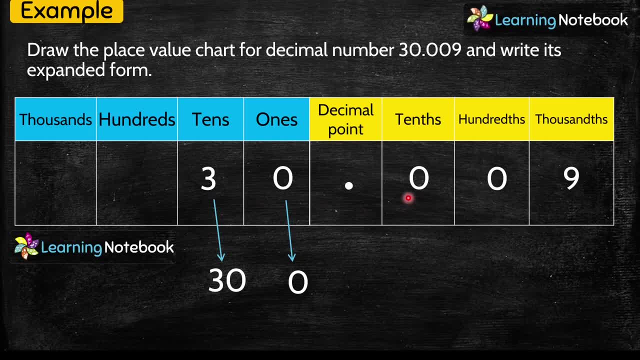 Now let's find the place value of the decimal part. Place value of this 0 will also be 0.. Students do remember that place value of 0 always remain 0, irrespective of its place. So place value of next 0 will also be 0.